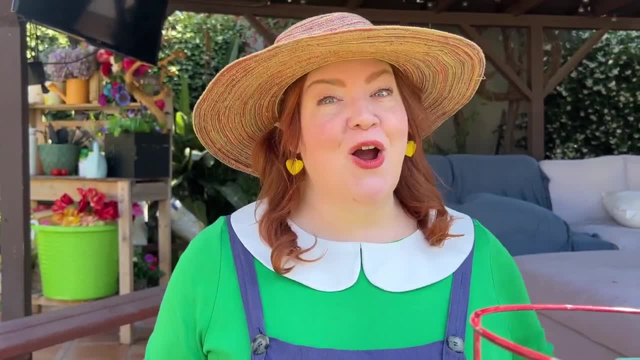 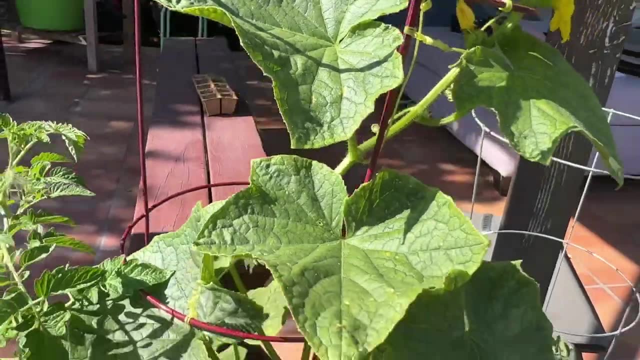 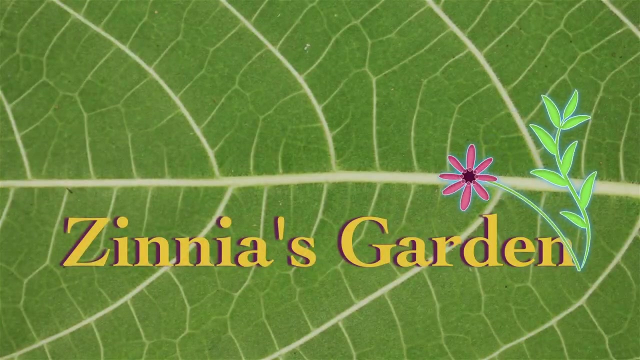 You don't need much to plant your own garden. All you need are some seeds, a patch of dirt and a little patience, and you can turn this into this. Wow, Come on, let's go have some fun. It's early summer and that means a lot of you just started summer break. 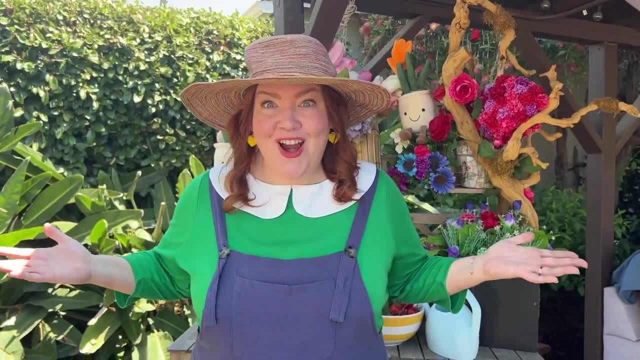 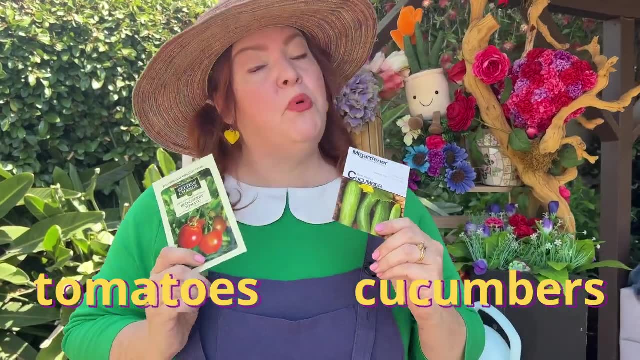 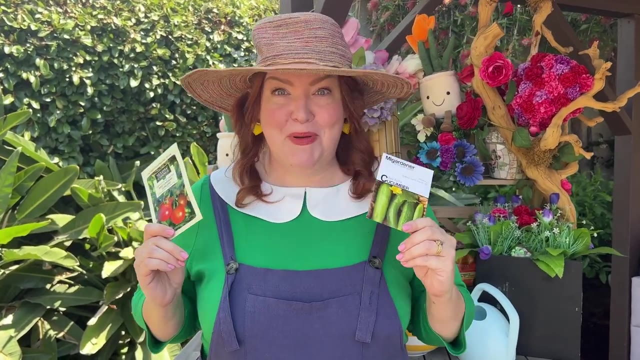 which is the perfect time to plant a garden. So today we're going to be planting cucumbers and tomatoes. Both of them grow very fast and you can plant them at the end of spring or early summer, when the weather starts to warm up a bit. You know what? Let's also plant some marigolds. 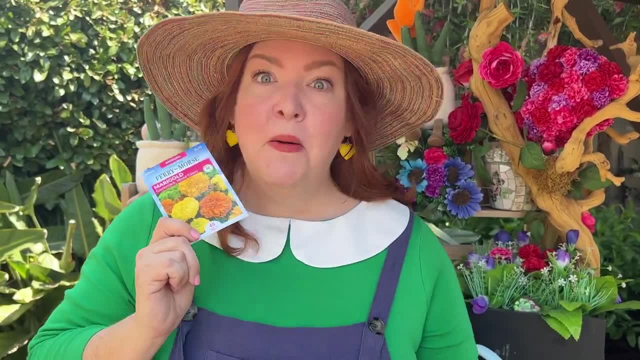 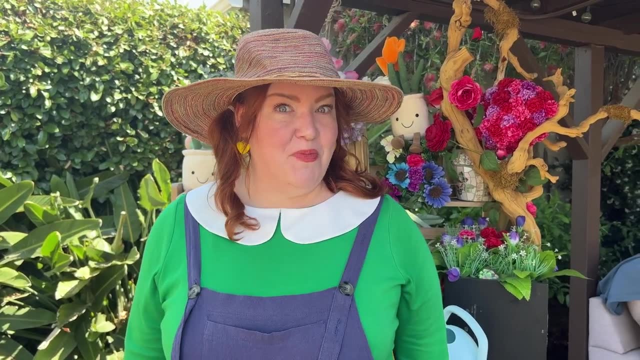 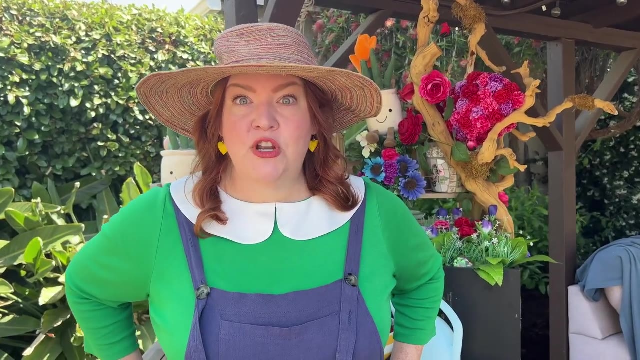 nearby. I love the smell of marigolds, but some bugs sure don't, which is great. Now that we know what seeds we want to plant, the first thing we have to do is decide where to plant them. Maybe you have a backyard, or maybe you live in an apartment. That's okay. 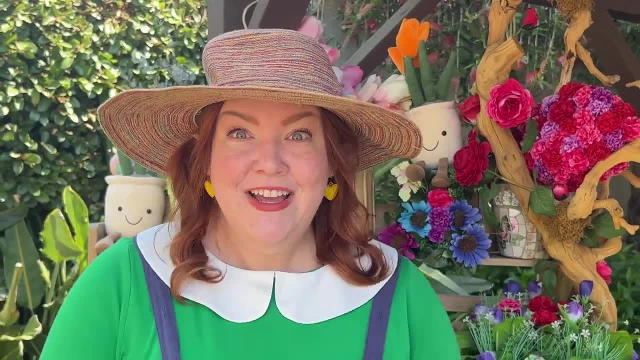 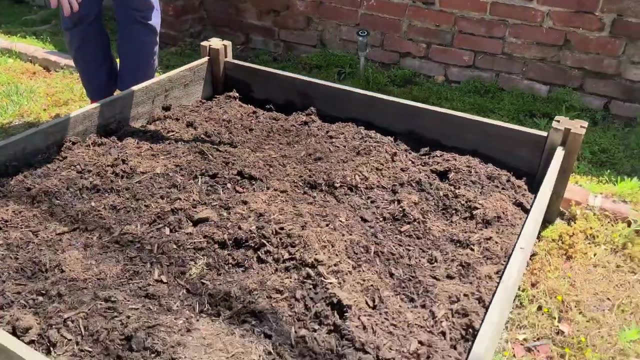 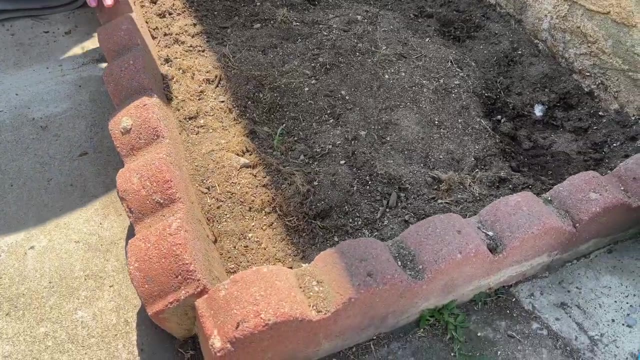 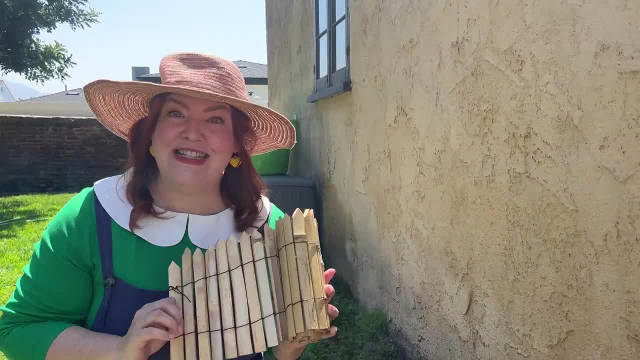 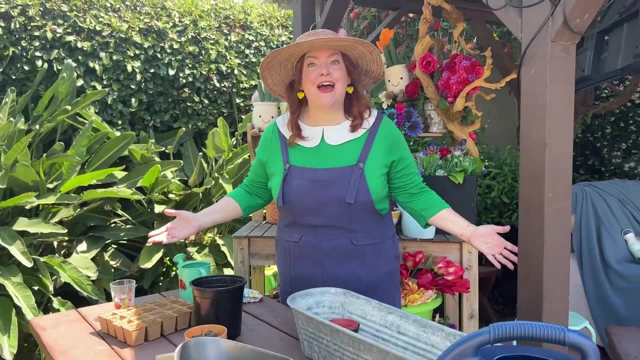 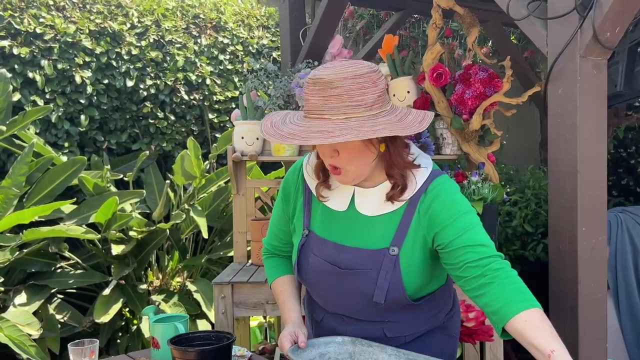 of wood. You can use a little bit of wood. You can use a little bit of wood to designate your area. I found this fencing at the 99 cent store And if you live in an apartment you may want to plant a balcony garden. You can use a long planter box like this and let your plants grow over the side. 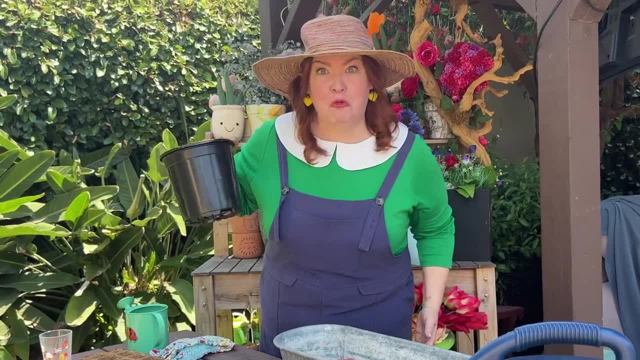 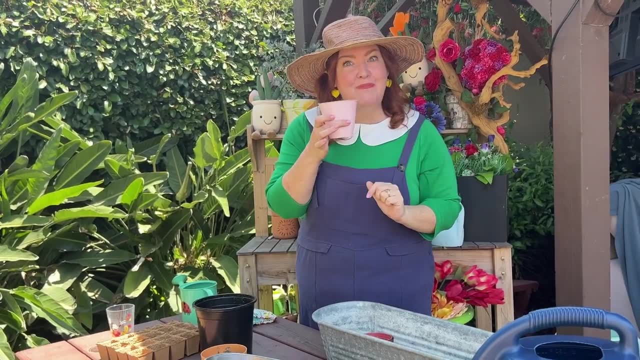 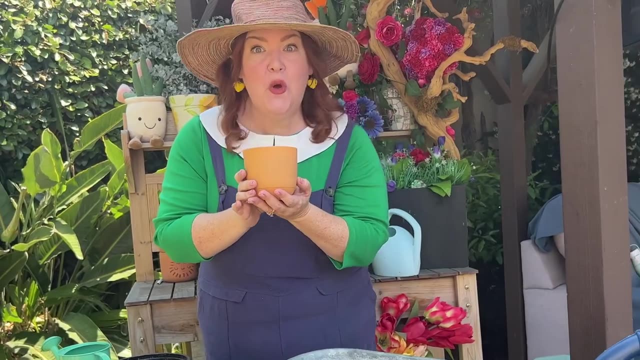 or you can use round buckets like this, even a real big bucket, just to grow your plants Or just to get started. you could even use this little cup- Just kidding. There's all kinds of receptacles you could use. You don't have to have a backyard. 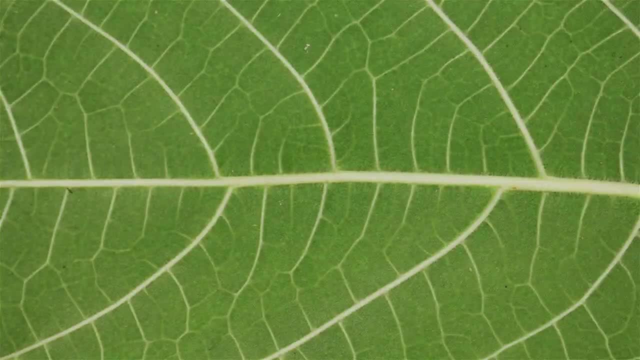 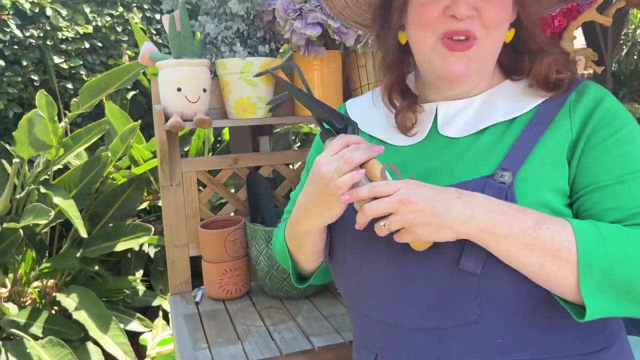 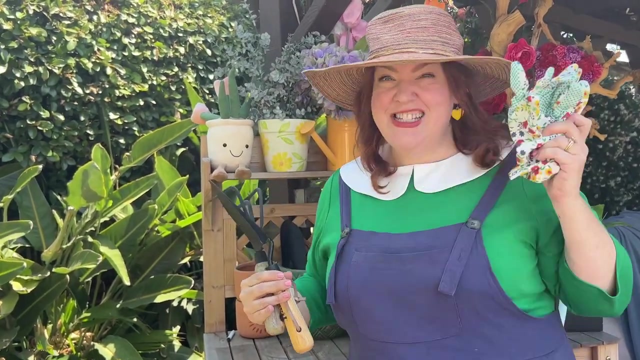 to make some seed magic. Small rake is handy to loosen up the soil, And let's grab a small shovel. You can find these tools anywhere: Walmart, Target, Dollar General, even the 99 cent store. And it's really handy to have a pair of gloves. And we can't forget. 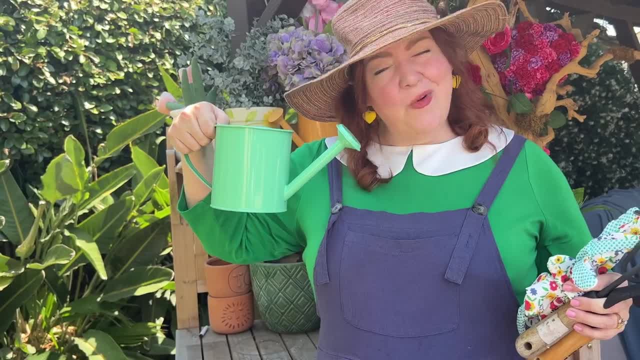 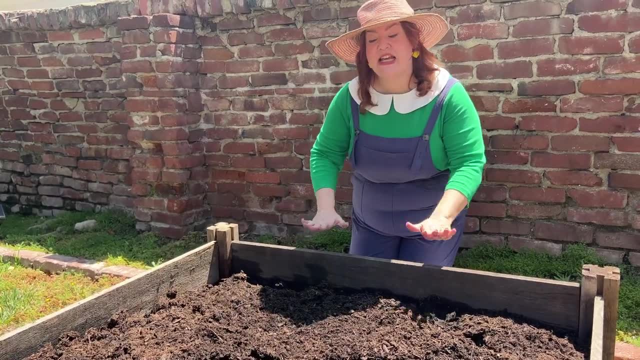 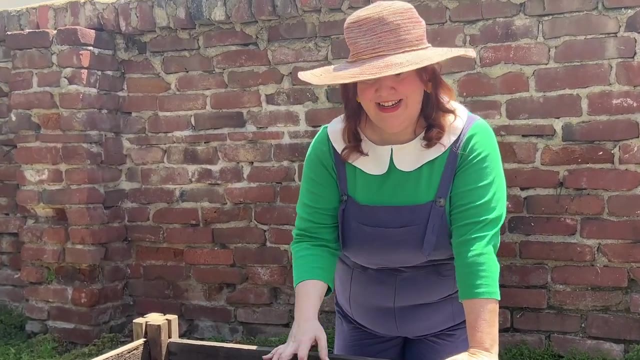 a watering can. Let's go garden. This is a raised garden bed that someone actually gave to me. Now this takes a lot of dirt. This is actually a mixture of outdoor potting soil and dirt from my compost bin. It's very healthy and ready to be planted, But if you're using a patch of dirt in your 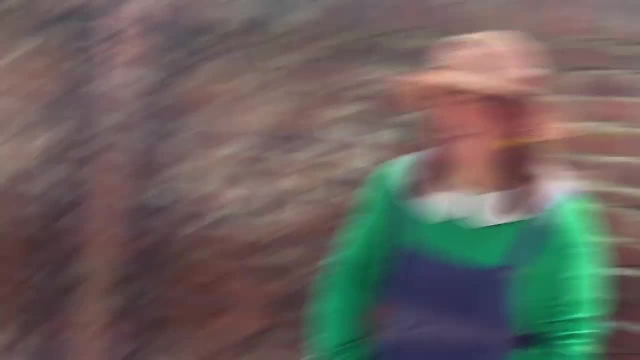 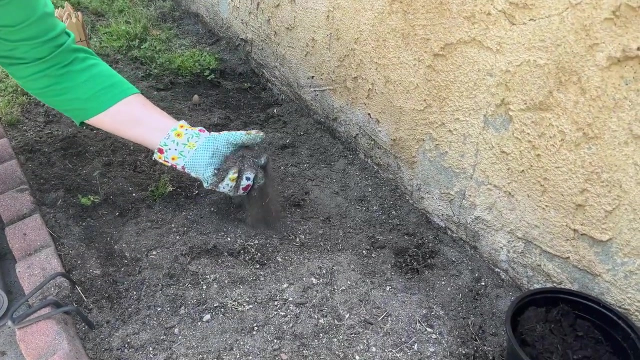 own backyard, we might have a little bit more work to do If you're not planting in a raised garden bed and you're putting your seeds directly into the ground. you want to make sure you have healthy soil. So let's check our soil. Is it dry and hard or is the soil loose? Get in there and loosen. 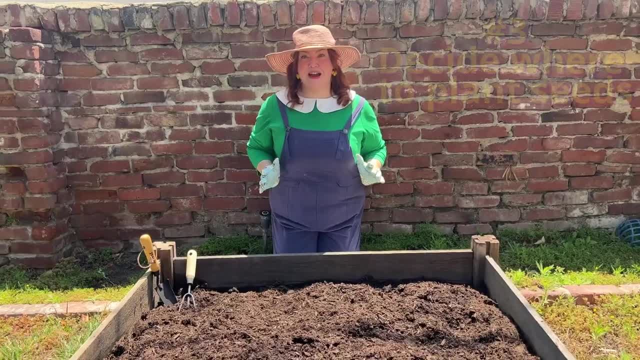 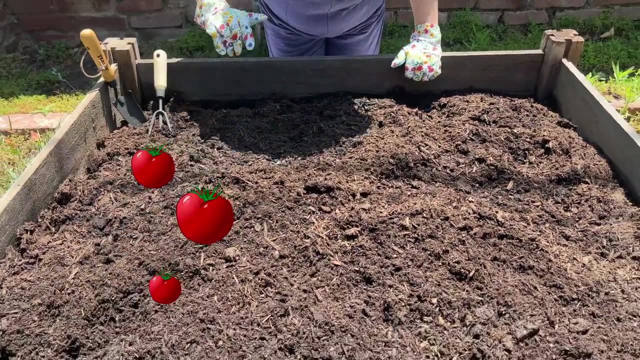 everything up, so your dirt is ready for planting. Now it's time to decide where we want to put each of our vegetables. So maybe we put tomatoes here, cucumbers here and marigolds right here, so everyone has room to grow. 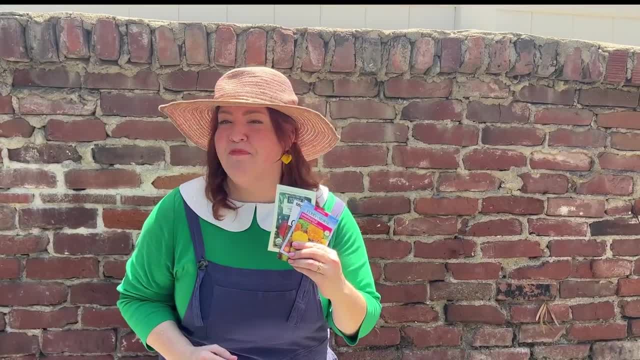 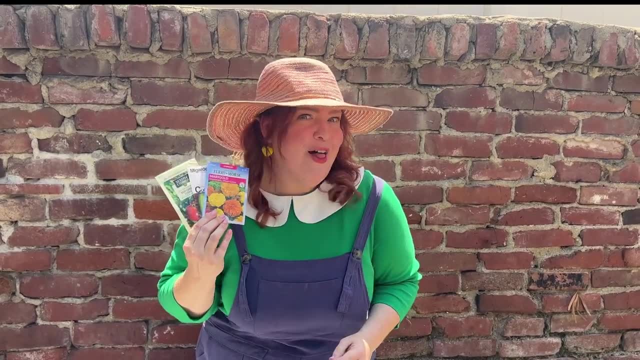 Next, it's time to plant. It's time to gather our magical seeds. You can find seeds anywhere at any store and they're not very expensive. I picked these up for $1.50, woo. Make sure to give each of your seeds. 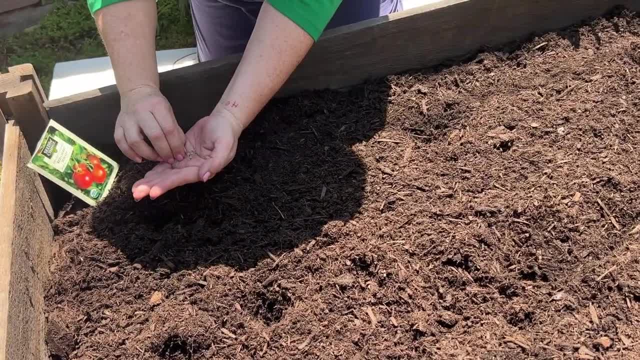 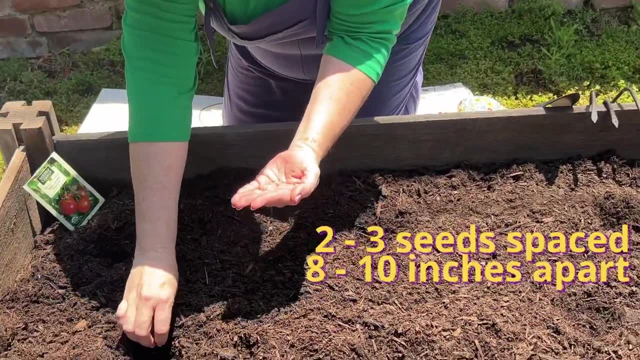 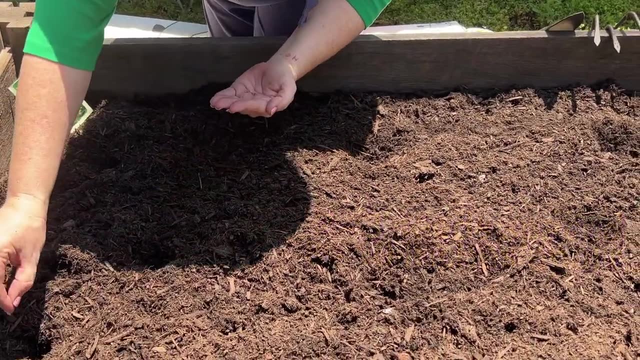 plenty of room to germinate. Now, with tomato seeds, you can actually put them straight into the ground. Take two or three seeds and drop them right in Eight to 10 inches apart. Plenty of space for these tiny seeds. Okay, little cucumbers, here you go. 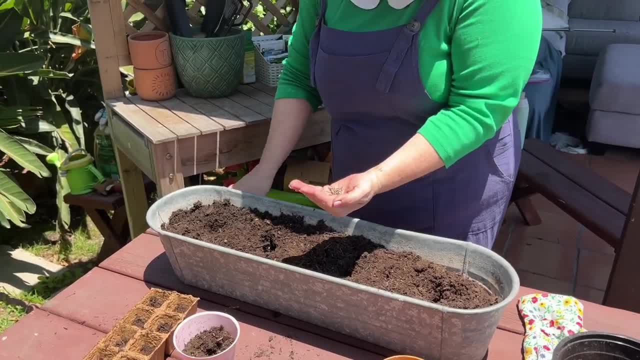 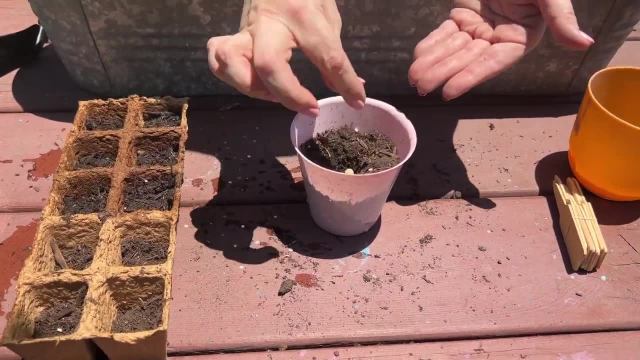 Remember same rules apply if you're using planters to start your garden: One type of seed per planter and space the seeds out so your seedlings have some breathing room, Deep breaths, little seeds and a quick row of marigolds.